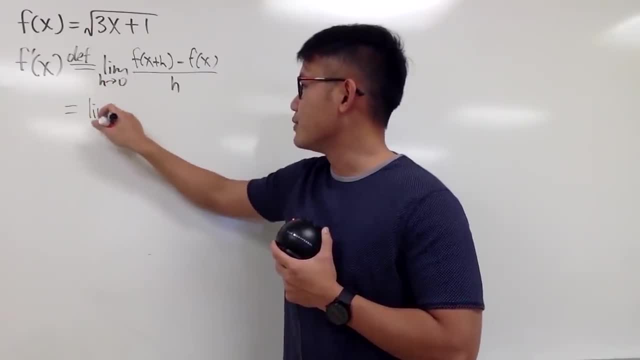 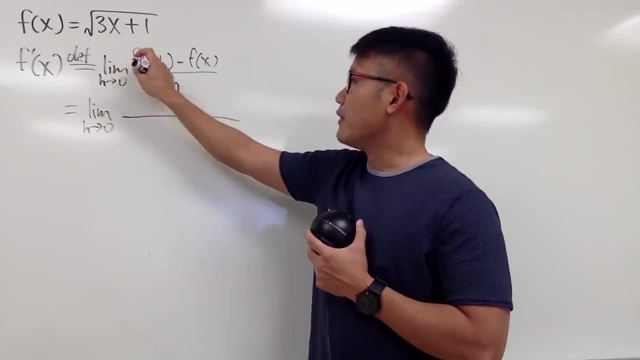 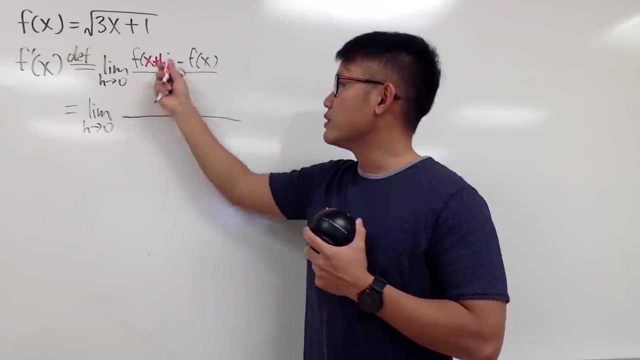 To continue, we get the limit And, yes, you have to just write down this as many times as we need to. Anyway, here, f of x plus h. This x plus h is our new input. All I have to do is to plug in this into this x. 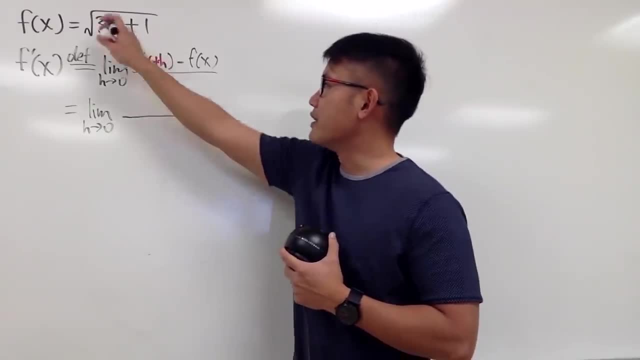 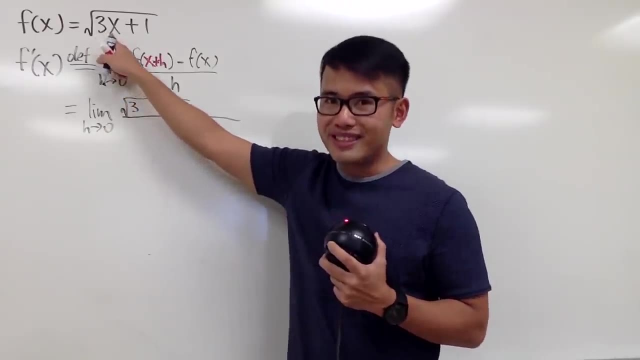 That's pretty much it. So for this part we will have the square root And then you have the 3 right here. But instead of this x, you open the parentheses and you put down x plus h. So we put down on parentheses x plus h, right here. 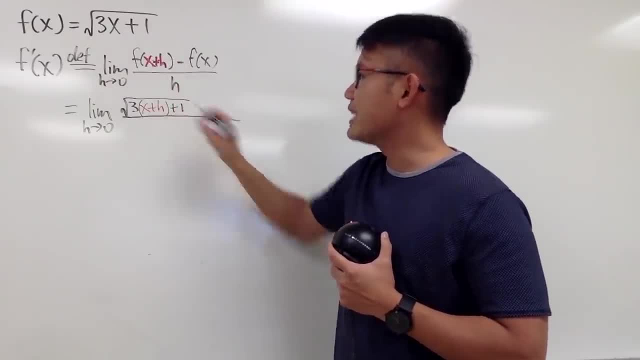 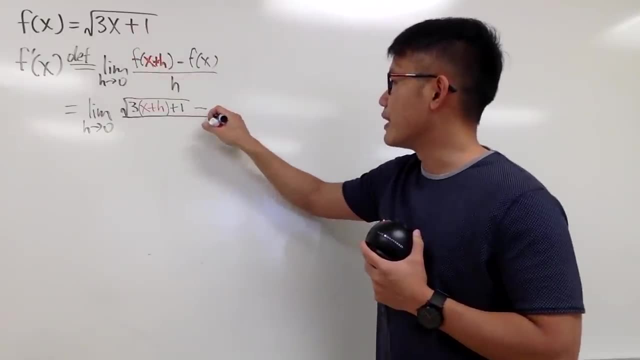 And then close that We still have the plus 1 after that. So that's it for that first part, And then you minus f of x, which is just that. So you just write down square root of 3x plus 1.. 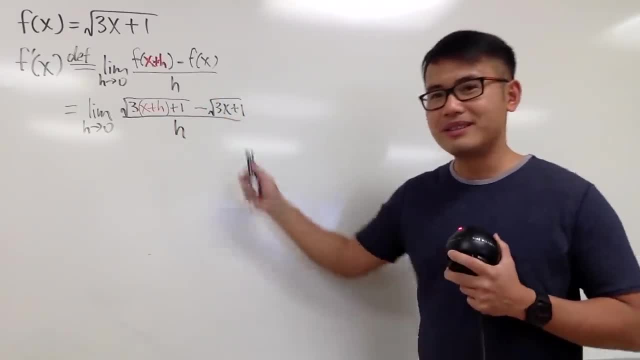 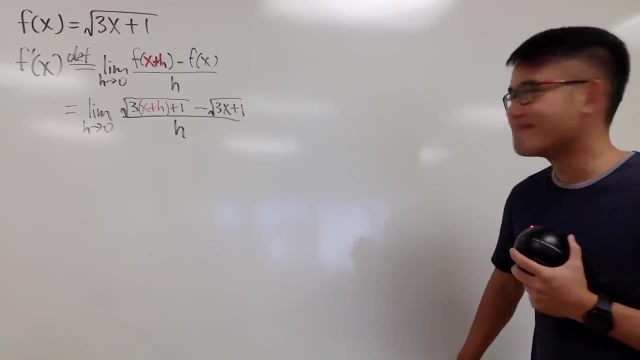 Everything, Everything over that h. So this is the setup, And now we just have to do some algebra from here to see if we end up with a nice expression or not. Okay, what can we do, though? Well, if you just plug in 0 into all the h, 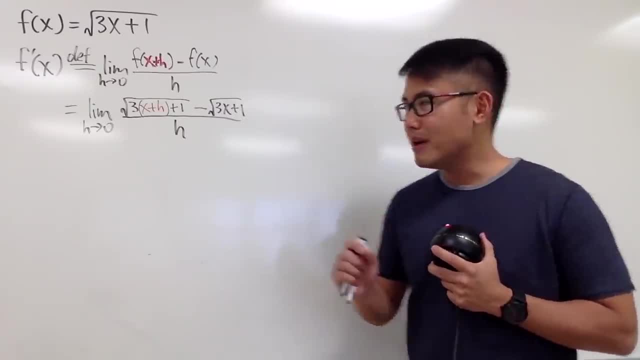 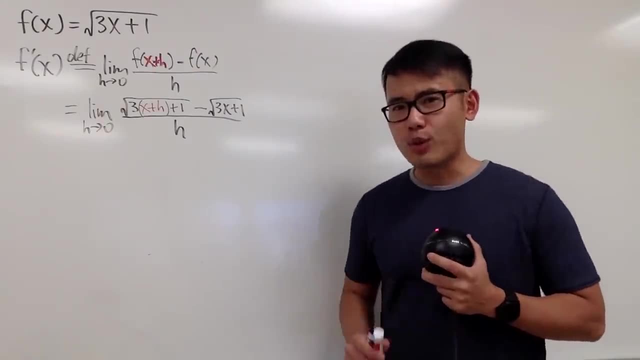 let me tell you, you end up with a 0 over 0 situation. We must do some algebra and some cancellation will happen, You'll see. Hmm, When we have square roots, what's the best thing for us to do? The answer to that is: 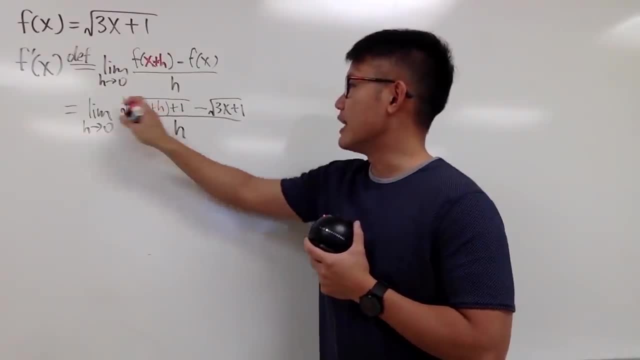 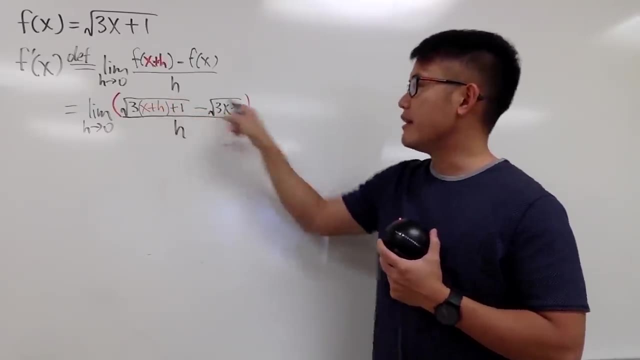 Use the conjugate right, And the conjugate of this is just that we will multiply the top and bottom Instead of this minus here. we will keep this and that the same, but you change that to a plus, So let me just multiply by square root. 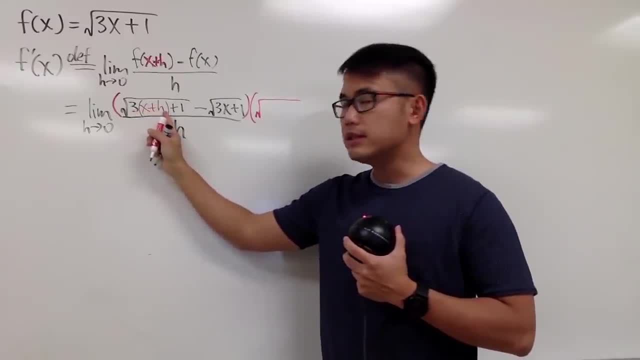 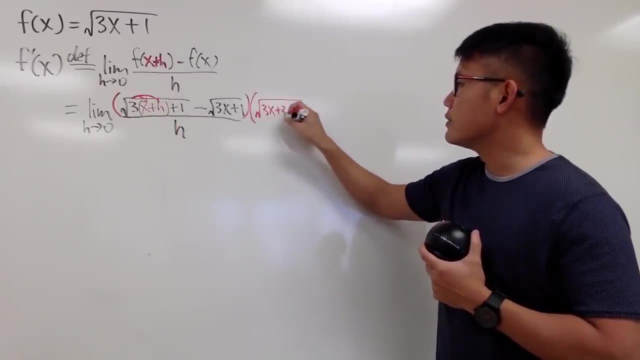 And, of course, notice that here we have the 3 in front of this parentheses. We should just multiply this in. So for this right here, let me just write it down as 3x plus 3h, And then you still have the plus 1.. 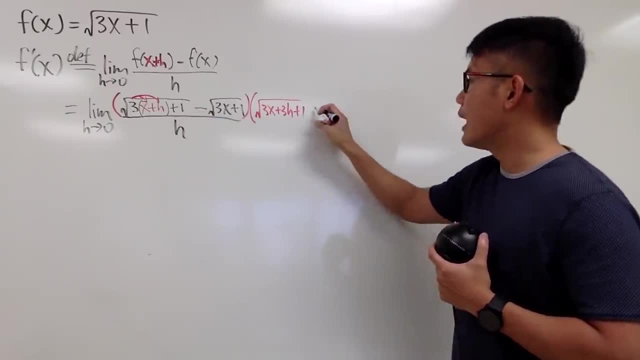 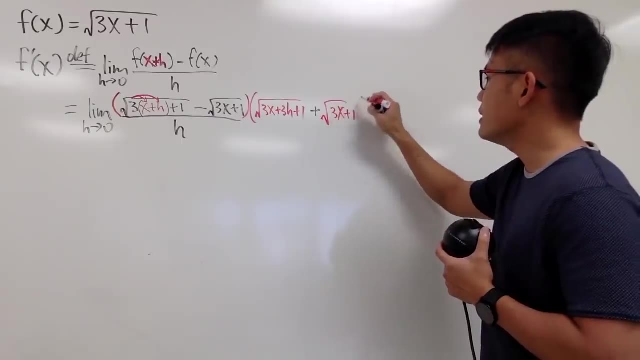 And instead of the minus you have to have a plus for the conjugate. And then this stays the same again: 3x plus 1.. So that's the conjugate, And you do it on the top, You do it on the bottom as well. 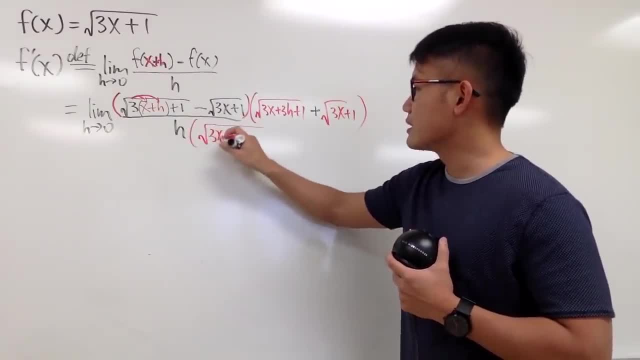 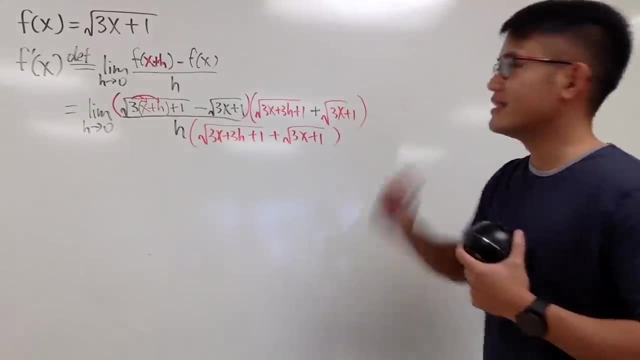 So let me just put this down: 3x plus 3h plus 1.. And then plus square root of 3x plus 1, like this: And we just have to do some algebra from here. Hmm, what can we do? 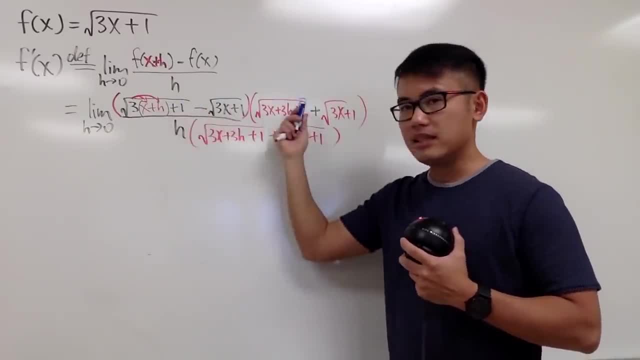 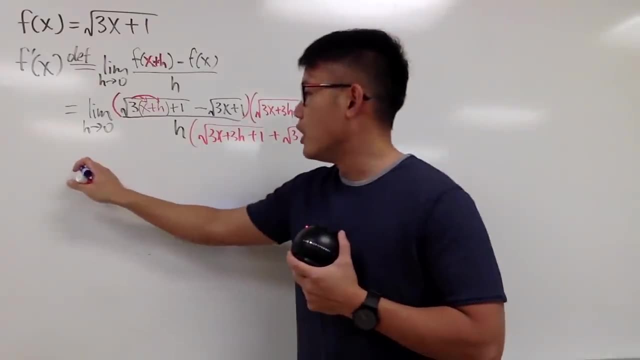 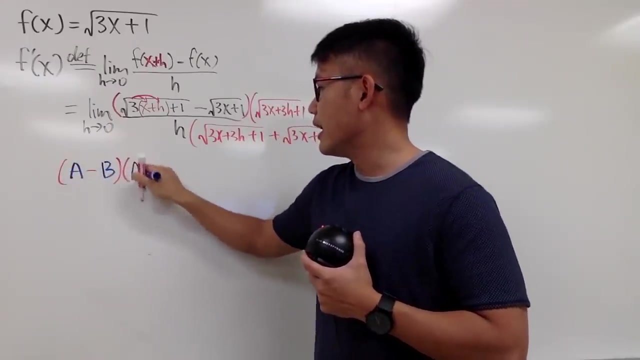 The beauty of using the conjugate is that this is in the form of a minus b, times a plus b. There's a nice formula for us to use to simplify this, And let me write this down. Whenever we have a minus b, and then we are trying to multiply this with a plus b. 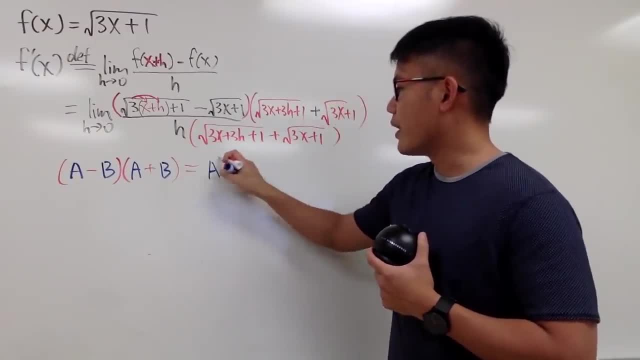 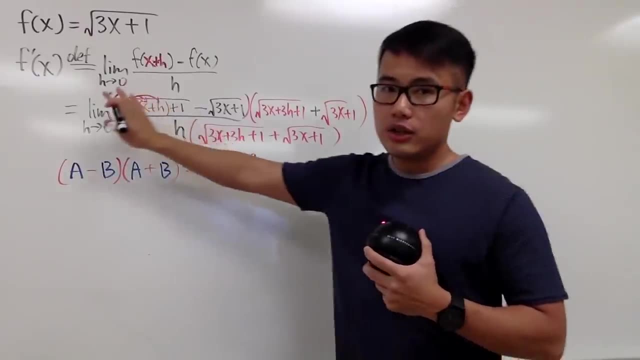 This right here: you just do a squared and then you minus b squared, That's all, And you will see it's really nice. So from here let me just focus on the top. This is equal to the limit, as h goes to 0.. 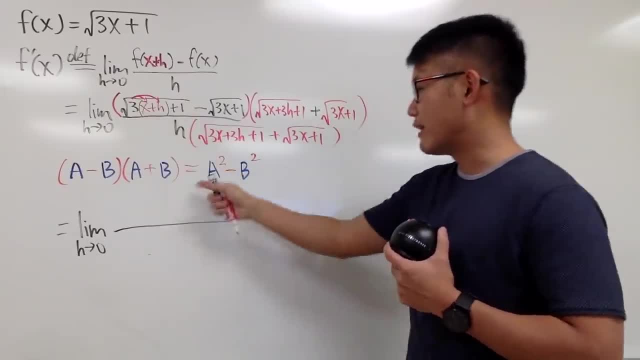 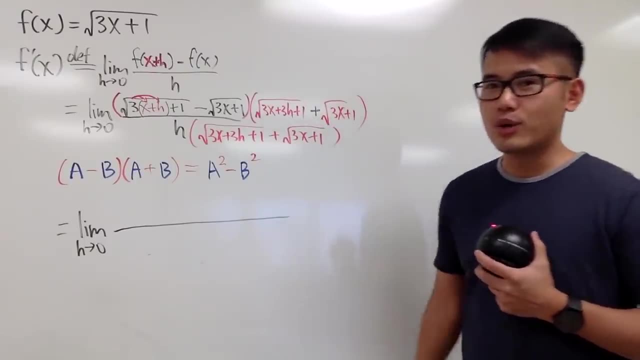 On the top. once again, this is the a but you just have to square that. And whenever you have the square root, you square that. You just pretty much cancel them out. The square root and the square cancel each other out. 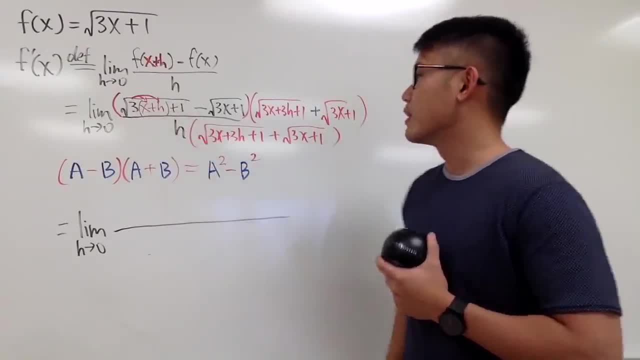 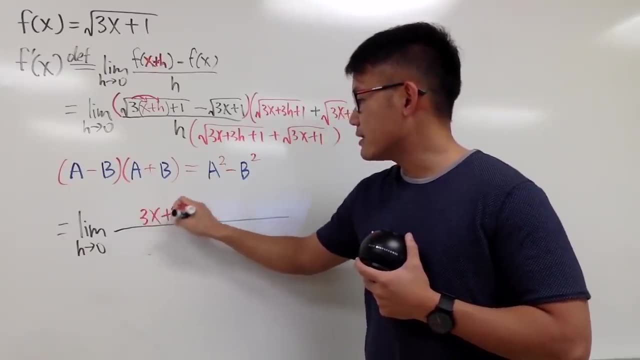 So, in another word, you just have the inside right here, first right, And this inside is the same as this inside, And let me just put that down: 3x plus 3h plus 1.. So that's the first part. 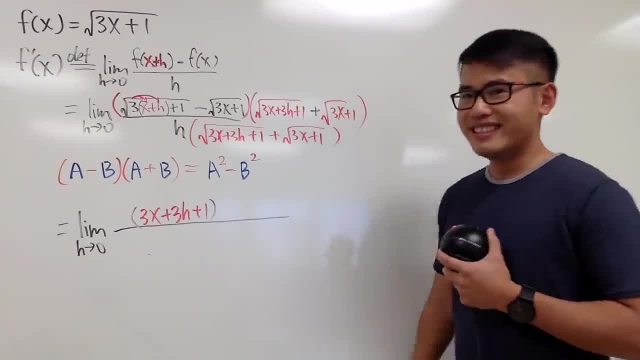 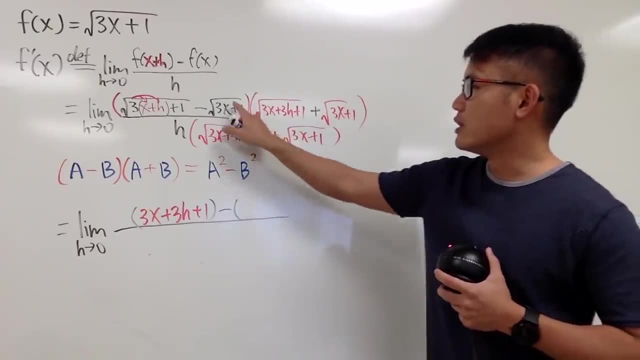 This time I will just put down parentheses: No more square root. And this is like the a squared part And next you minus The second part is b squared. which is this thing squared Once again, square root, cancel out. 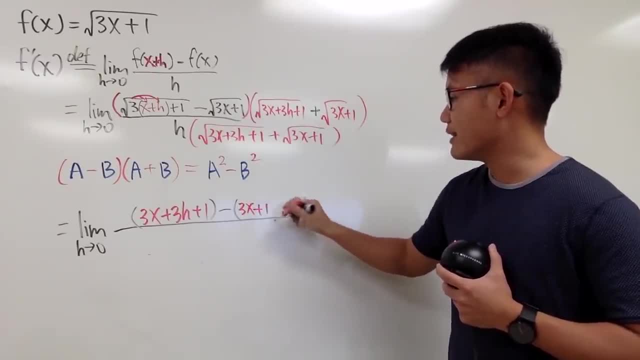 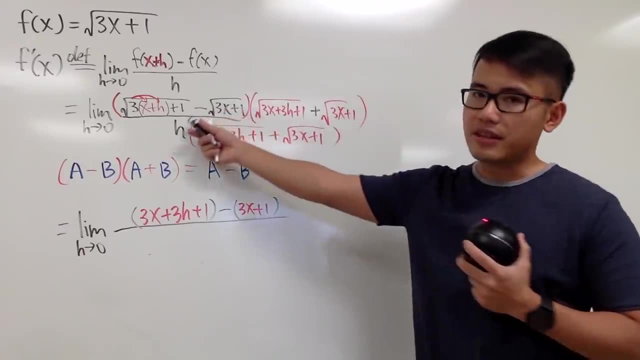 You just have the inside. I will just write down 3x plus 1.. So that's the top, And here is something you should keep in mind. The reason that we're using conjugate is to fix the top right And then we multiply it out. 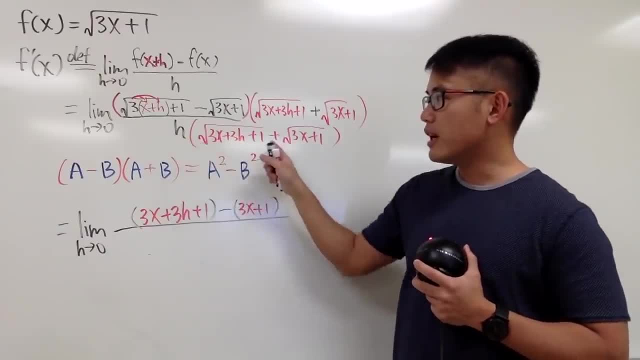 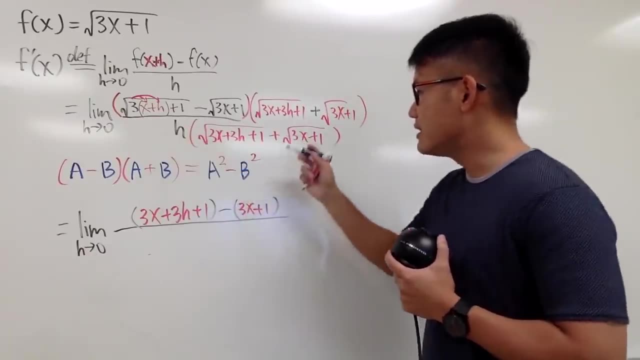 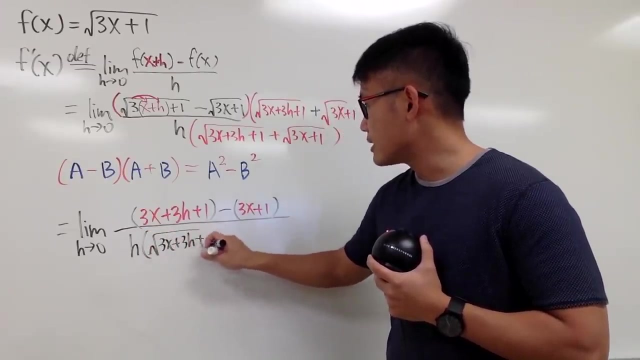 This is what we have ready And the conjugate on the bottom. we are not going to multiply it out because you will see good things will happen in a minute, So I will just write this down as how it is: h times parentheses: square root of 3x plus 3h plus 1. 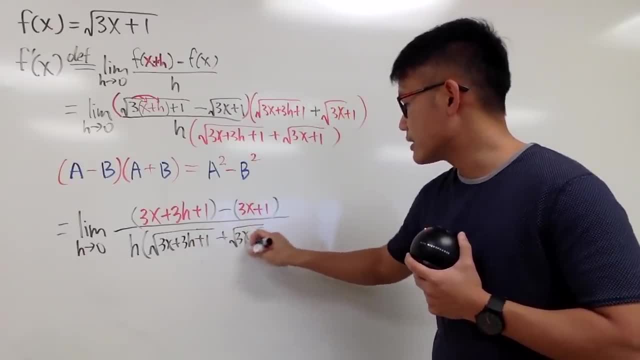 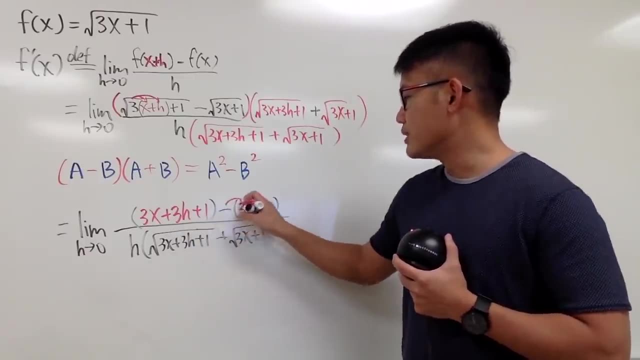 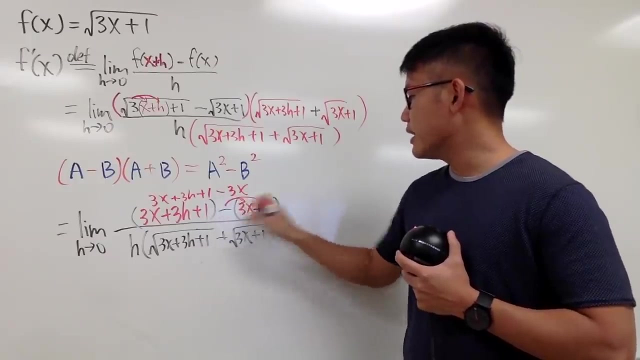 and then plus square root of 3x plus 1.. Well, we just have to Fix the top a little bit more Notice you can just distribute this into the parentheses, So you get pretty much 3x plus 3h plus 1 minus 3x and then minus 1.. 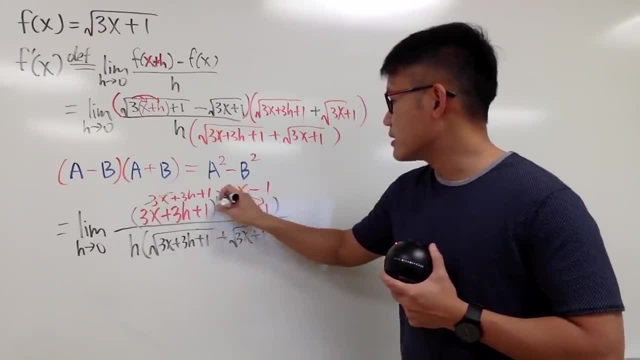 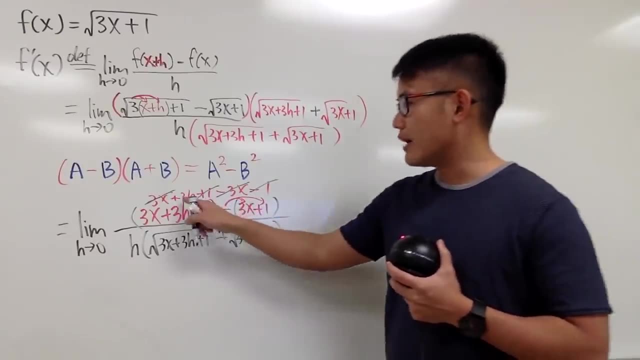 And what happens? 3x minus 3x? of course, they become 0. Likewise, 1 minus 1 is also 0. So you pretty much have 3h on the top And on the bottom. you notice that you do have this h. 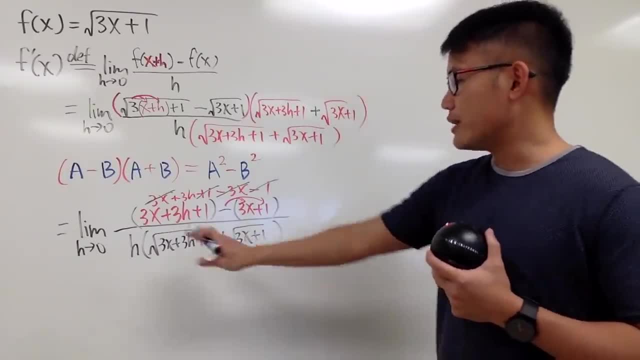 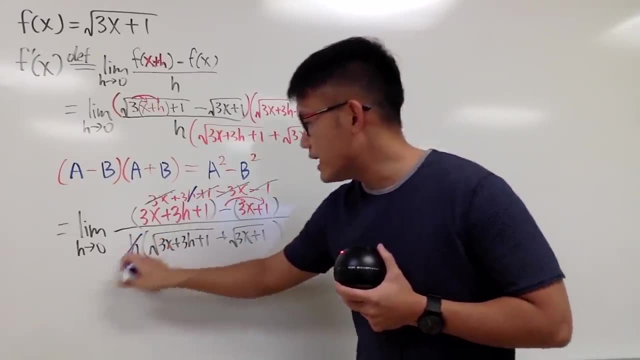 And that h you can cancel. So it depends if you want to write this down again or not. We can just cancel out the h right here And I will do that for you guys. I'm going to cross out this h with that h. 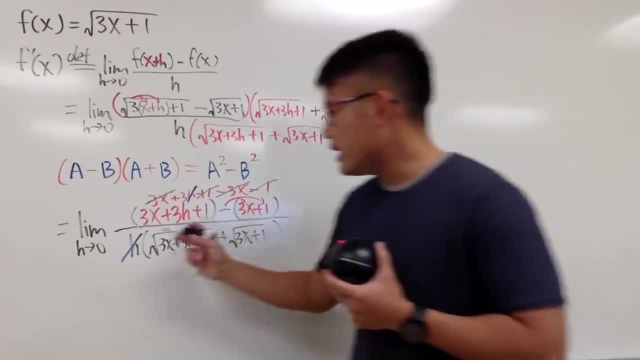 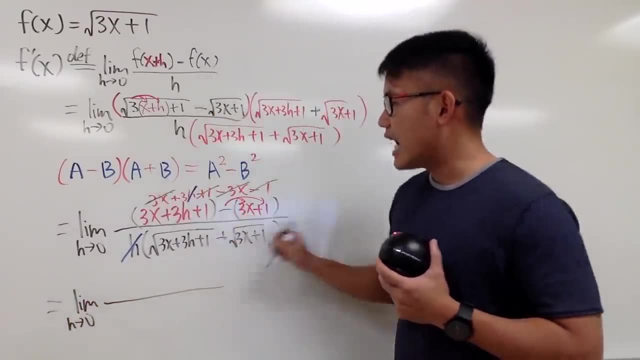 So this is pretty much the simplification. In the end, we see that this is nothing but just the limit, as h goes to 0. On the top, you just have this 3 left, okay, And then this h is also gone. 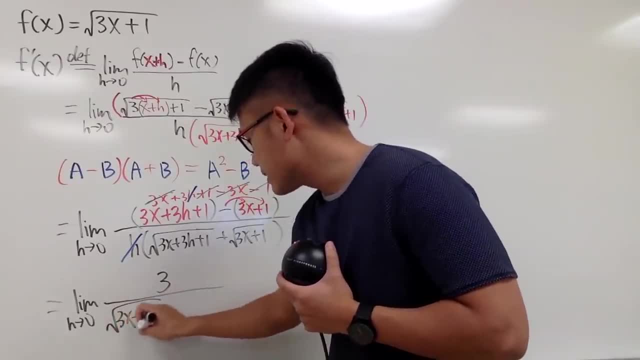 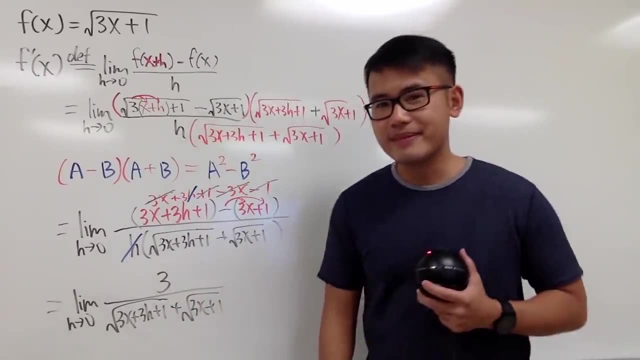 So we just need to write this down: Square root of 3x plus 3h plus 1, and then plus square root of 3x plus 1.. And notice this, and that when they cancel out, in fact you cancel out the 0 over 0 situation. 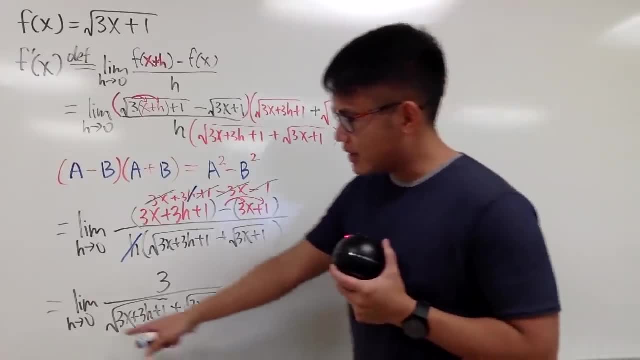 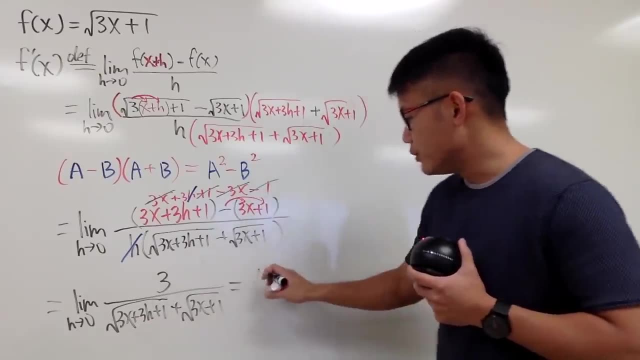 And that's so wonderful, Because now you can just plug in this 0 into this h and you get the next answer. So I will show you guys the work. for that You get 3 over. This is square root of 3x plus 3 times 0. now 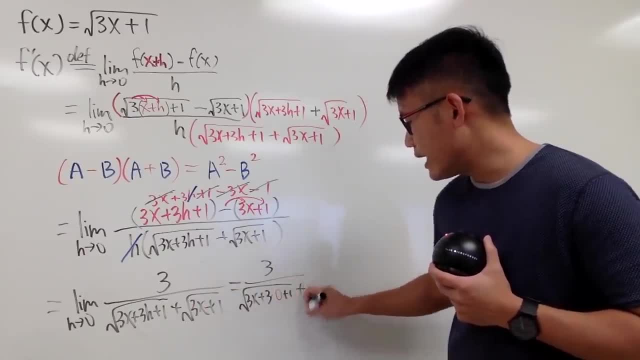 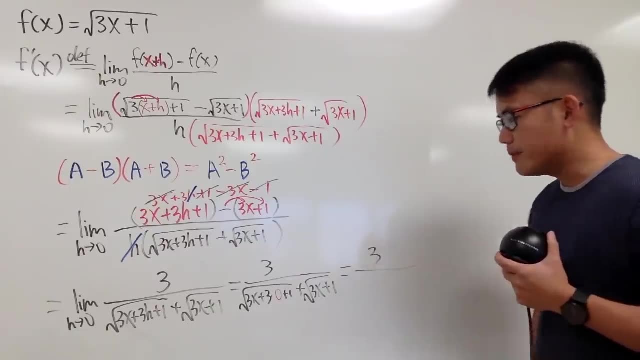 And then you add 1, and then you add this one again, which is square root of 3x plus 1.. And you see that on the top is 3 over. Notice this: 3 times 0 is just 0.. 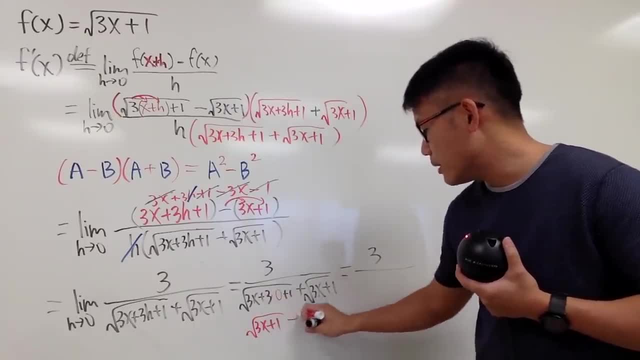 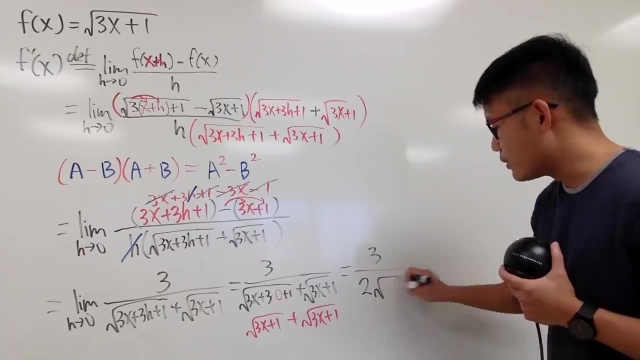 So you pretty much have square root of 3x plus 1 plus another one, Two of this, and they are the same inside, So of course you can combine them. In fact, you get just 2 square root of 3x plus 1.. 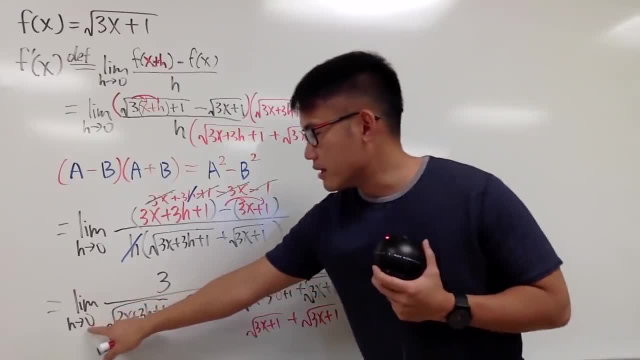 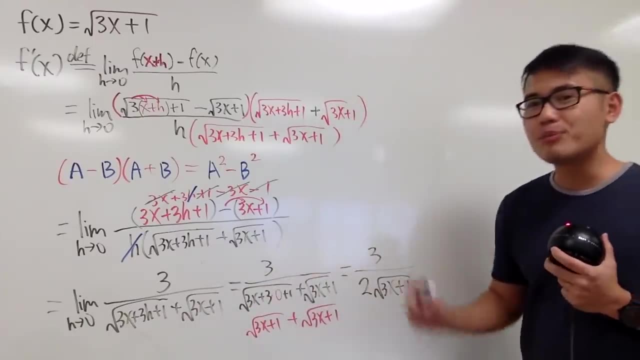 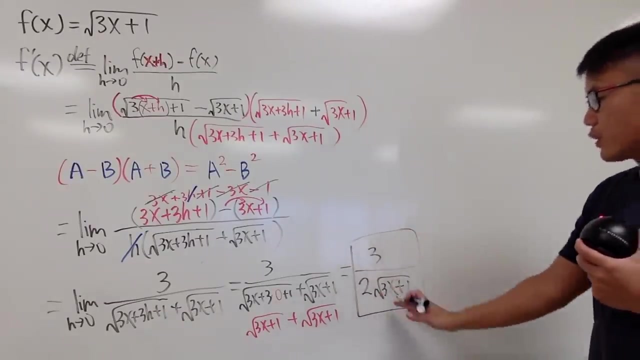 And this is the answer. And notice, when I plug in the 0 into this h, I didn't write down limit because I took the limit already. This is the computational part for that And this is the final answer. Namely, we get 3 over 2 square root of 3x plus 1.. 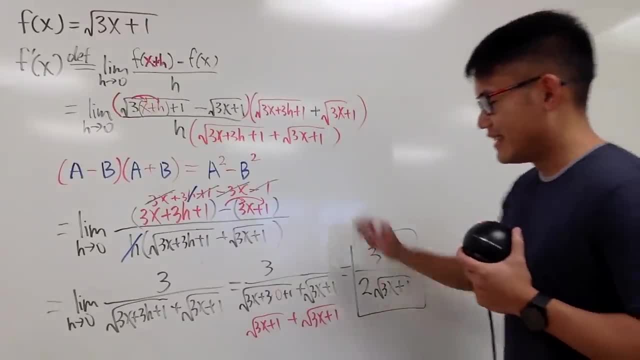 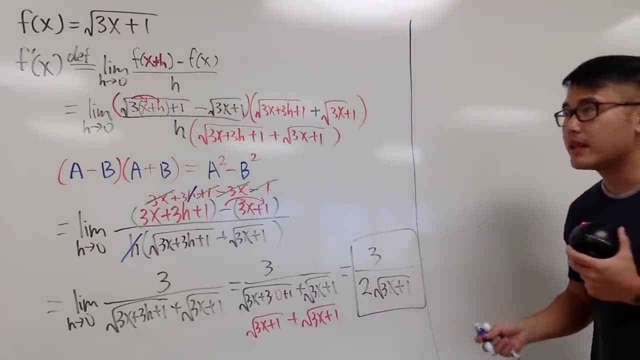 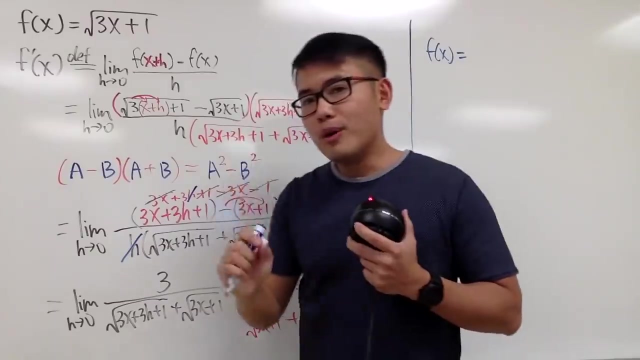 And that's the derivative of this function. So this is the good definition of derivative, And now let's talk about how we can possibly do it in a shorter way. So let me write. Let me write this down again: This is f of x equals to almost always, okay. 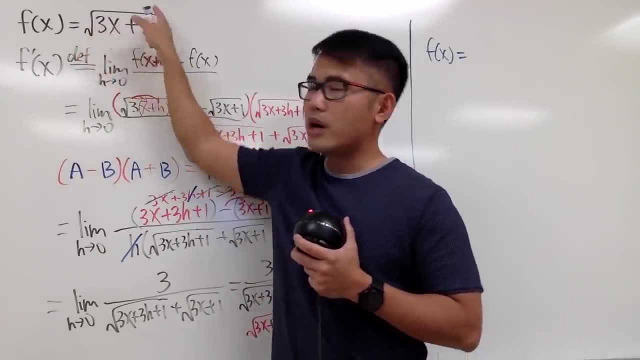 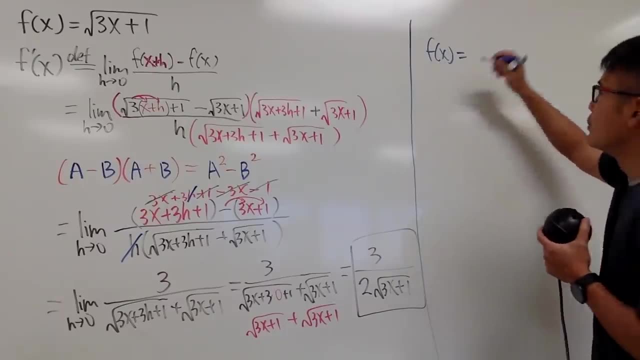 Keep this in mind. In calculus you almost always look at the square root as 1 half power, So I will just write that down for you guys. In other words, f of x is equal to parentheses 3x plus 1 inside, raised to the 1 half power. 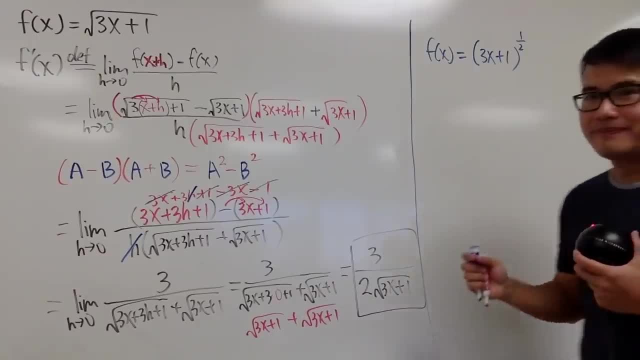 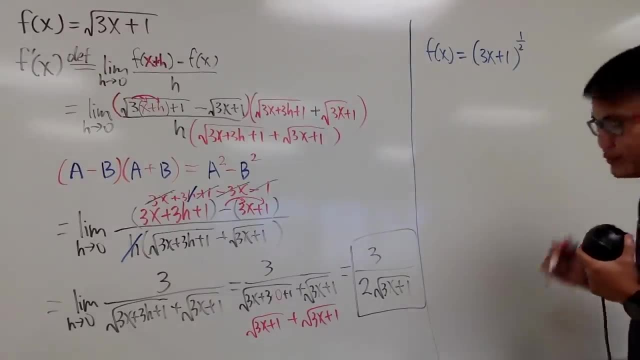 Why? Because when you have the power form, you can use the power rule, Everybody's favorite method- right. Well, do this one really really carefully. First of all, let me just write down f, prime of x for the derivative. 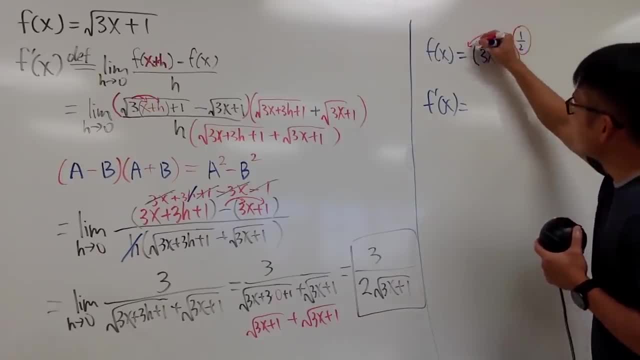 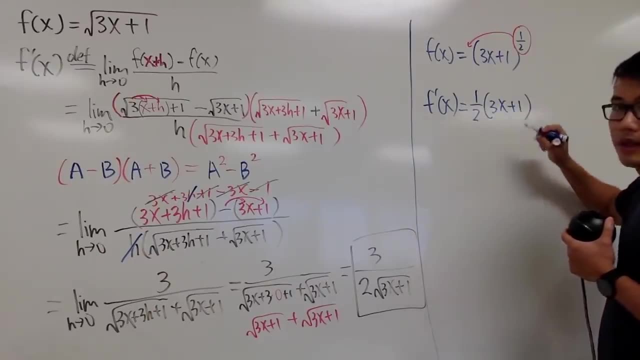 Right here, I will just circle the power and bring that to the front. So you just have the 1 half And then the inside stays the same, 3x plus 1.. So you bring the power to the front And then you have to minus the power, right here. 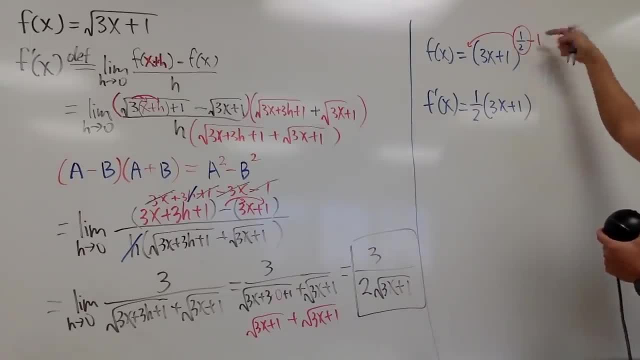 This is going to give you the new power. So 1 half Minus 1.. This is negative 1 half. now And let me just put this down for you guys to see what happens: This is raised to the negative 1 half power. 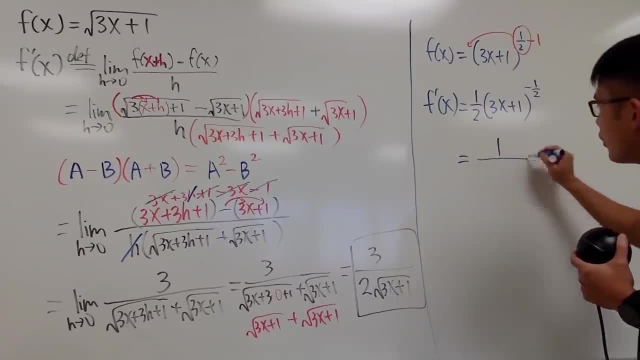 In other words, we can bring this down to the denominator And this will join these two in the denominator, So we have 3x plus 1. And then the 1 half becomes positive, And then you can of course write this back as a square root. 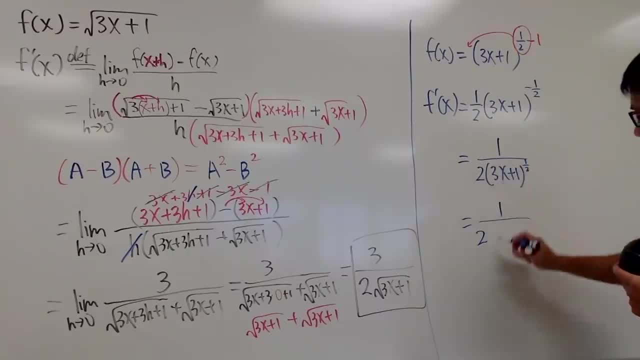 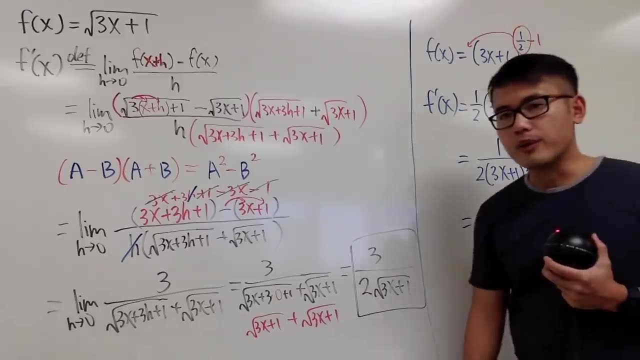 So this is just 1 over 2. And this becomes a square root Of this 3x plus 1.. And you see, yes, I used the power rule And this is the answer that I got for the derivative. 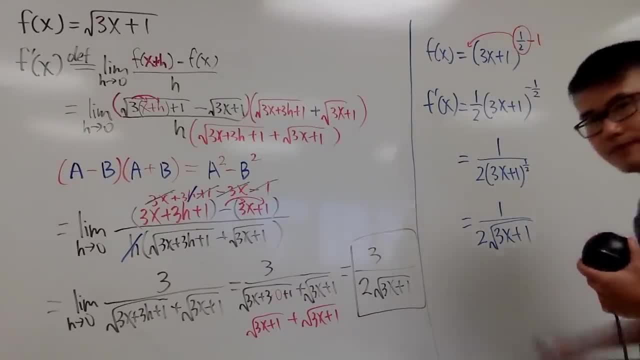 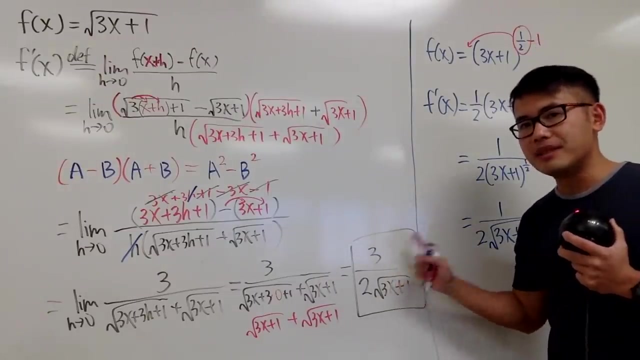 But what happens? What's wrong? Well, this is certainly not the same as this. And what's the difference? Yes, on the top here I have 1.. But by using the definition of derivative, we saw that this right here should have been a 3, right. 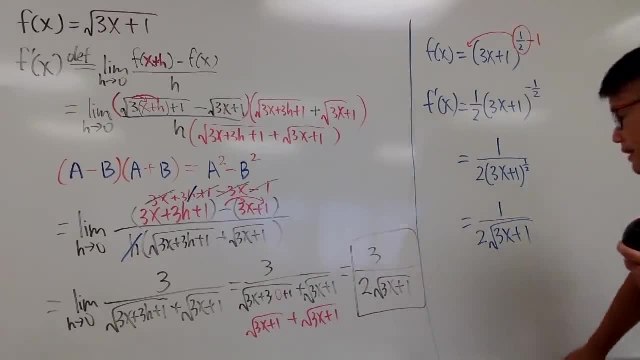 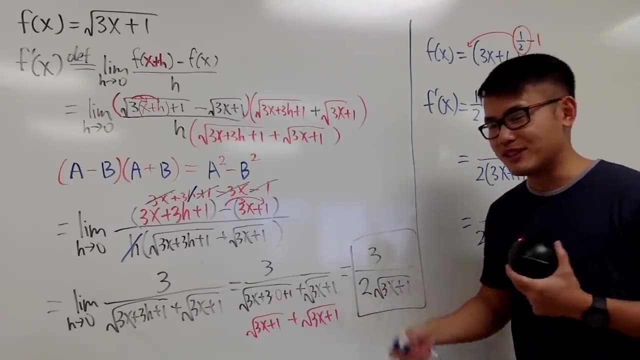 But I don't think we've made any mistake. So this is the time that you have to remember, And this is how I like to point out the chain rule situation with my students. Imagine you just do the power rule which we did. 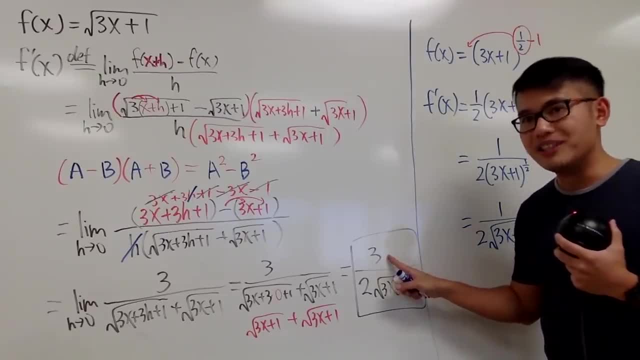 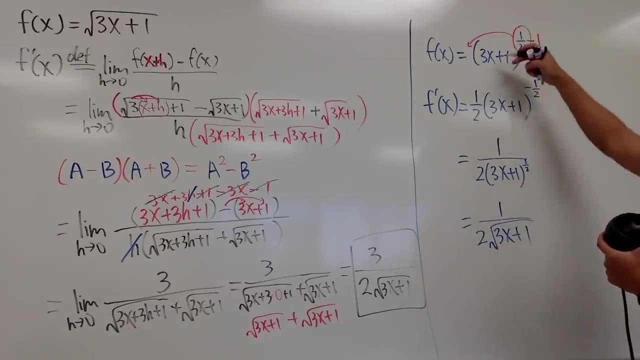 How in the world can we multiply by this 3 legitimately? And the answer to that is: we have to think derivative. Notice this 3 is pretty much the derivative of the inside. You see the inside here. So the derivative of 3x plus 1 is precisely this 3.. 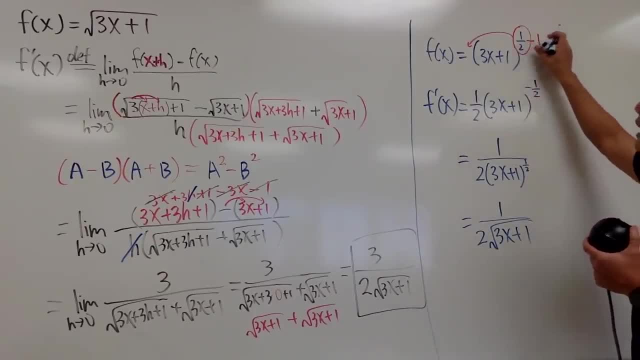 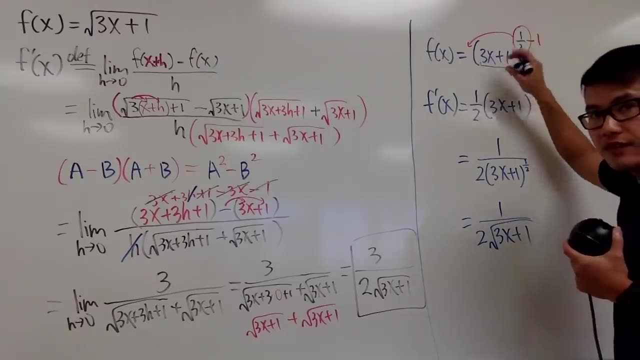 So what you do- the power rule is what you do right here- is that after you do the power rule, you go to the inside function and then you ask yourself what's the derivative of the inside function, which is just this: 3?.